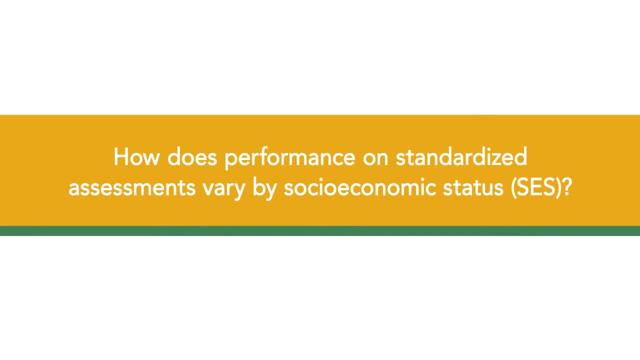 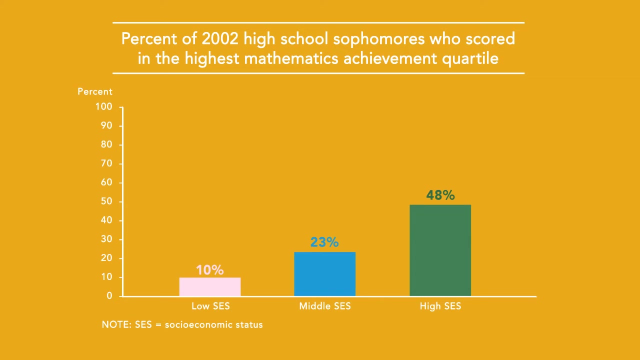 In order to make comparisons, NCES divided the students in the national sample into four groups based on mathematics achievement. while in high school, In general, a smaller percentage of low SES students performed in the highest mathematics achievement quartile, while in high school, compared to middle SES students and high SES students. 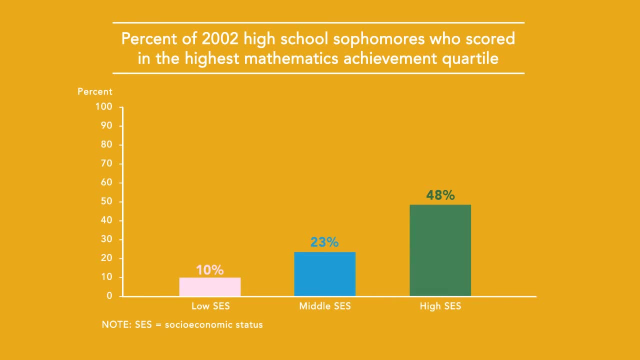 Overall, 10% of low SES students were in the highest mathematics quartile, compared to 48% of high SES students. On the other hand, a larger percentage of low SES students performed in the lowest mathematics achievement quartile while in high school, compared to middle SES students and a larger 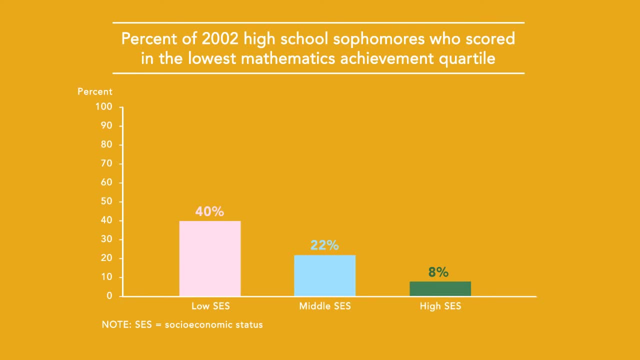 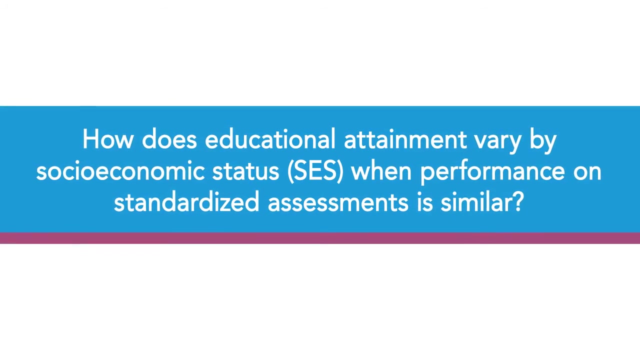 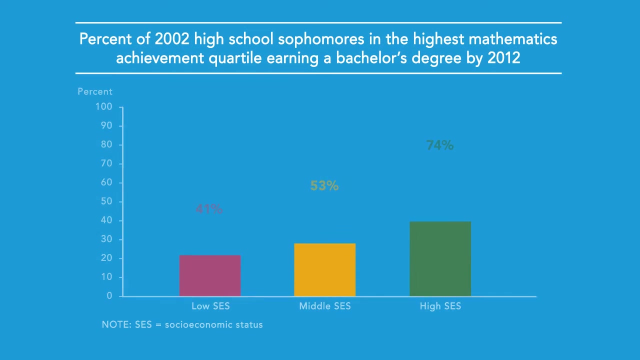 percentage of both low and middle SES students performed in the lowest mathematics achievement quartile while in high school, compared to high SES students. Now let's examine how educational attainment varied by socioeconomic status. when performance on standardized assessments was similar For students who scored in the highest mathematics achievement quartile: 41% of low SES students. 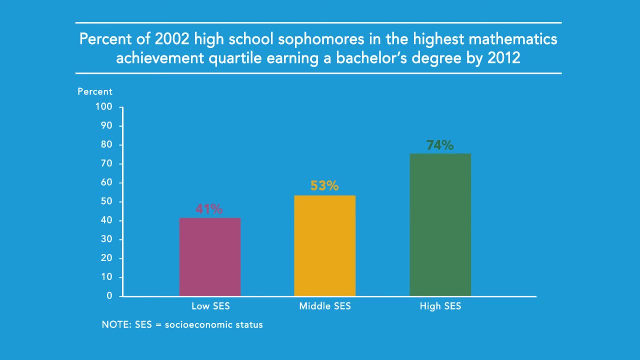 had completed a bachelor's degree in 10 years, compared to 53% for middle SES students. The latter is the lowest score among the students with the highest achievement quartile, while in high school, If one student scored in the highest math quartile, they would become a high SES student. 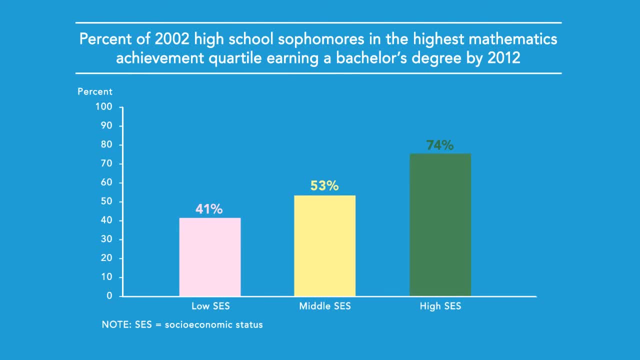 middle SES students. These percentages were both lower than the 74% of high SES students who had completed a bachelor's degree. Now let's compare these completion rates with those who scored in the lowest mathematics achievement quartile: Only 5% of the low SES students who scored in the lowest 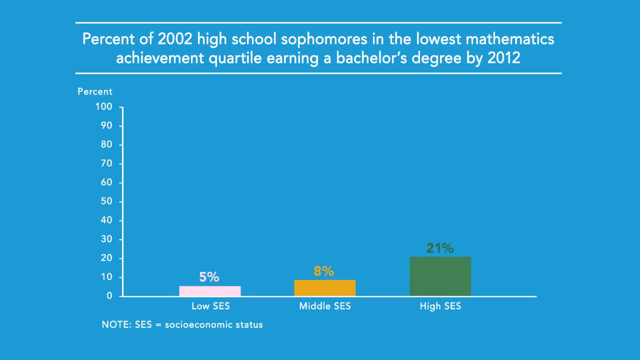 mathematics achievement quartile in 2002 went on to complete a bachelor's degree by 2012.. This percentage was smaller than the percentage of middle SES students, and both of these percentages were smaller than the percentage of high SES students who completed a bachelor's degree by 2012.. Visit ncesedgov to 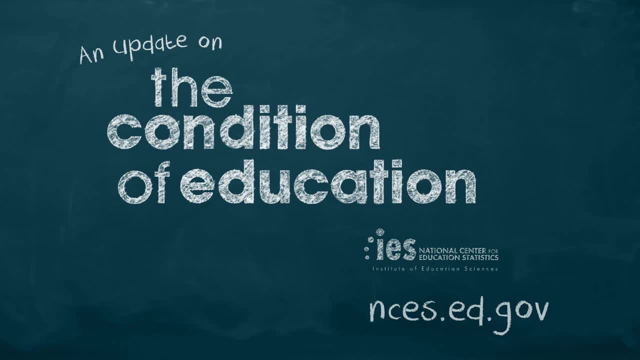 view the full report and learn more about the condition and progress of American education.